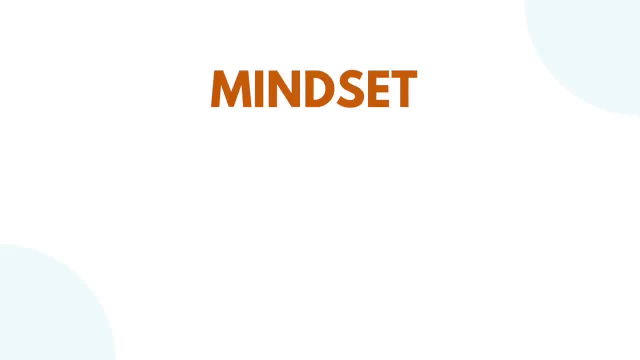 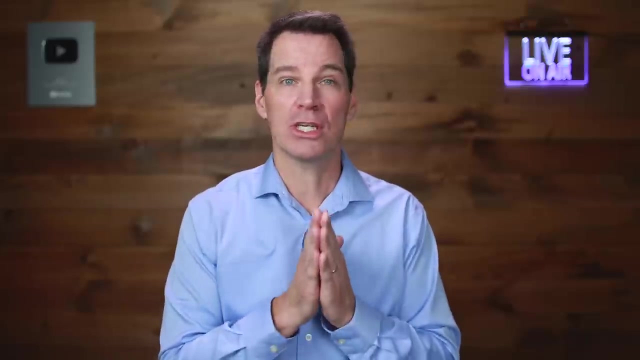 video. Like I said in the last video, working on our mindset is powerful, but it's only half of the story. We can also use behavioral strategies to reduce our nervousness and get this feedback loop moving in the right direction. So these six behavior changes can very quickly transform the 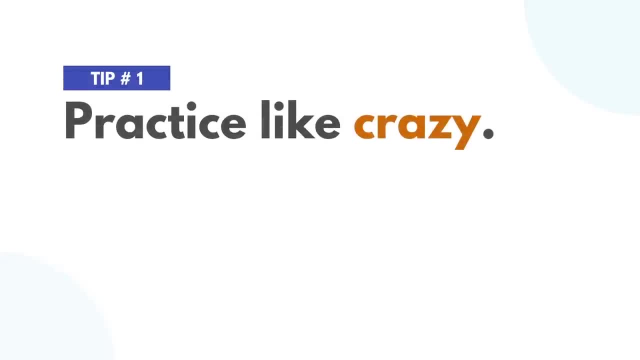 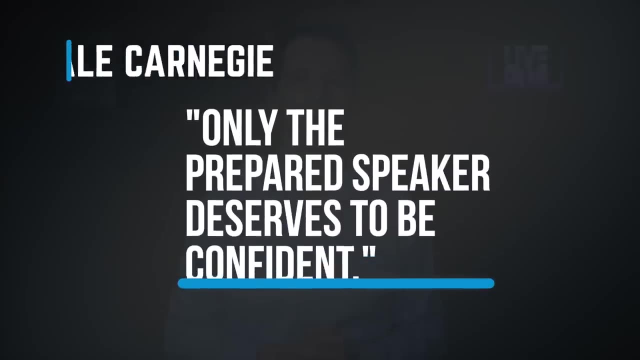 way you feel about public speaking. The number one way is to practice like crazy. Practicing is not a quick fix, but it's the best way to feel better. Dale Carnegie once said that only the prepared speaker deserves to be confident. I recommend practicing a presentation 10 times. 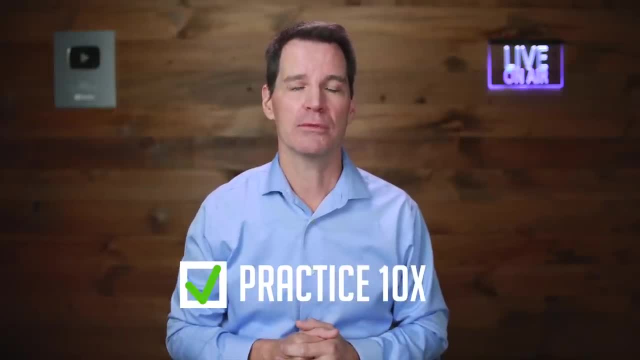 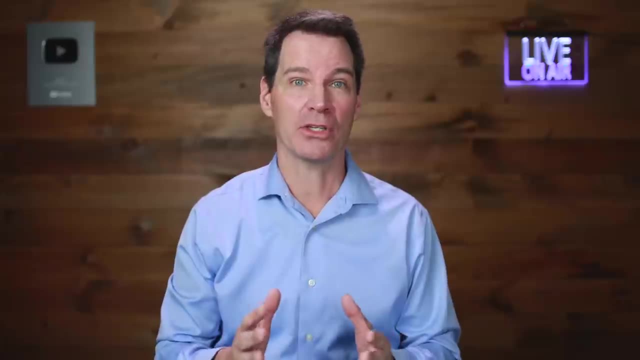 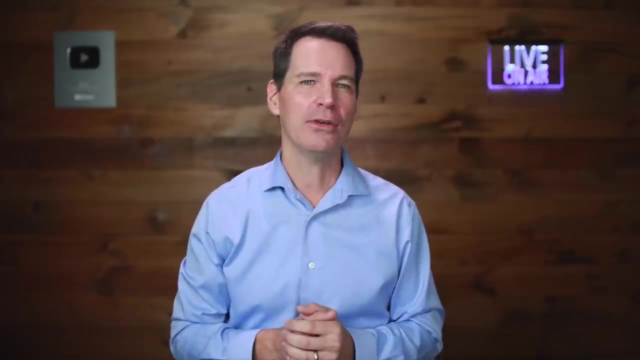 behind the scenes spread out over a few days beforehand to really let it sink in. Even if you still feel those butterflies, you can be confident that you are prepared. Trust in your preparation process: If you've already gone through the presentation 10 times in practice, now you're just going to do. 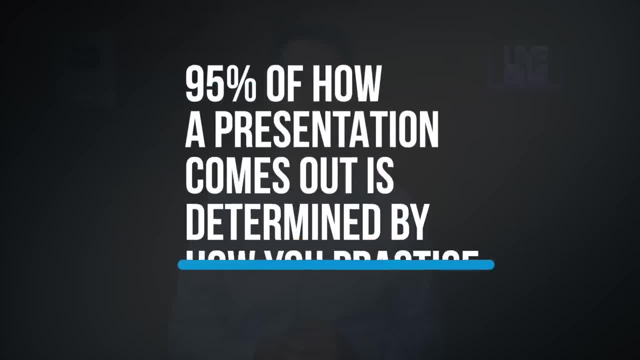 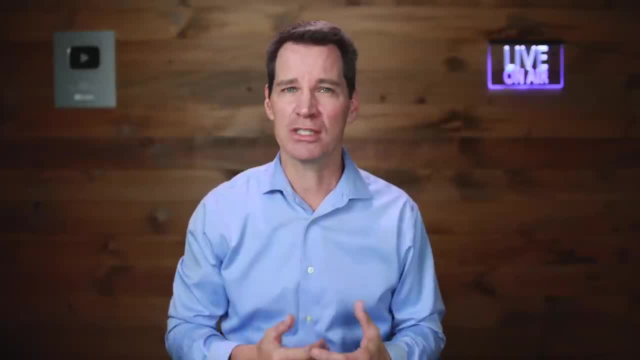 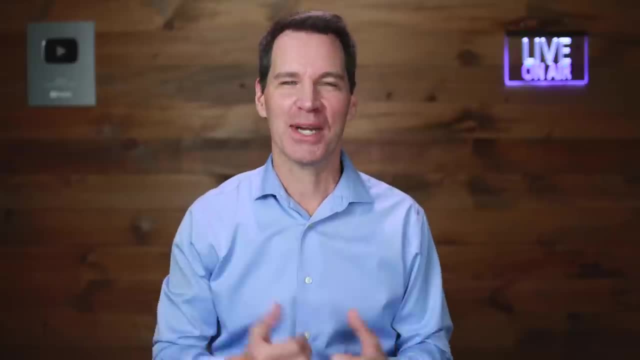 that presentation the 11th time And, as I've often said, 95% of how a presentation comes out is determined by how you practice. So even if you're still nervous, that won't stop you, as a prepared speaker, from doing a strong presentation. So practice like crazy and trust that process. 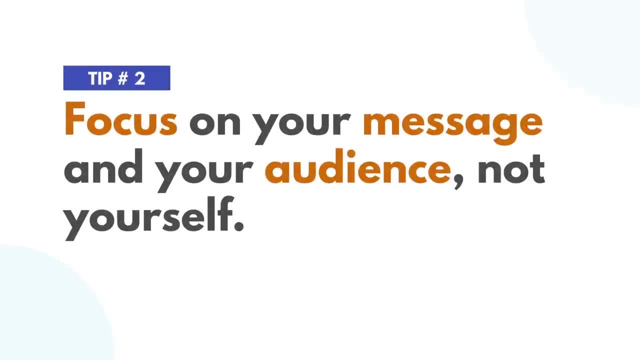 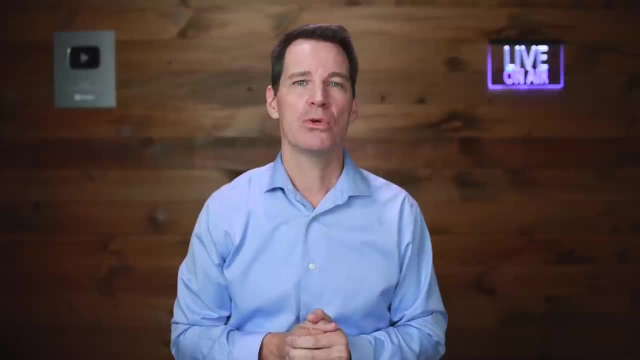 Number two: as you prepare, focus on your message and your audience. The three-part principle is to practice like crazy. Parts of a public speaking situation are the speaker, audience and message. Speakers, who get the most nervous, focus on themselves. What if I mess up, What if they don't like me? And when we? 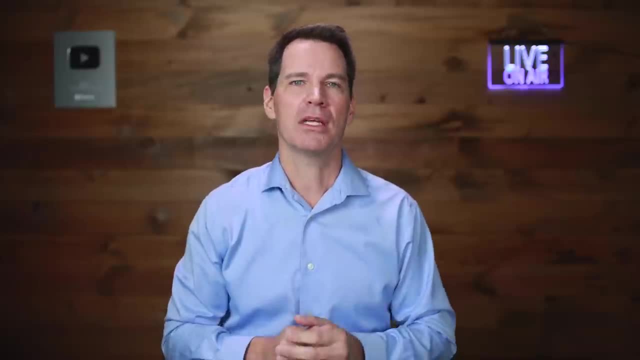 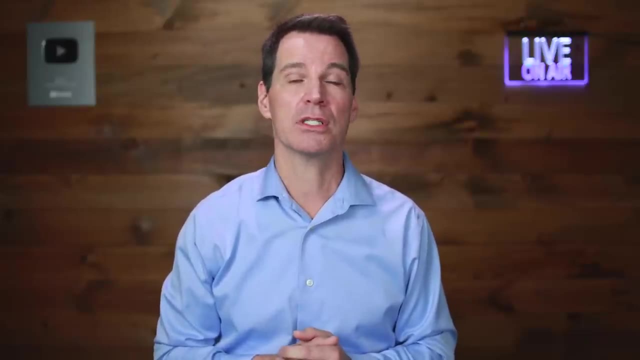 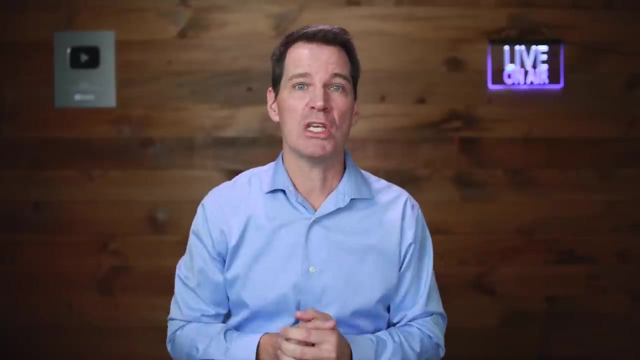 focus on ourselves and being perfect, we can psych ourselves out. I would say that perfectionism and that threat of feeling judged are the two biggest problems that we focus on, and that we're thinking about ourselves and most of that Instead. as you prepare and as you speak, 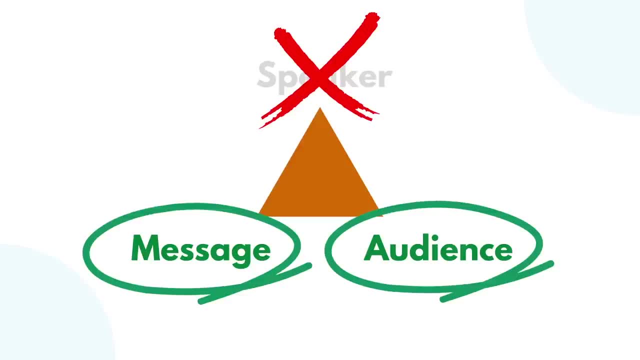 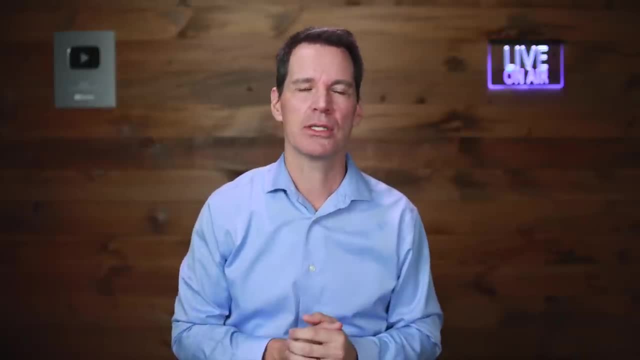 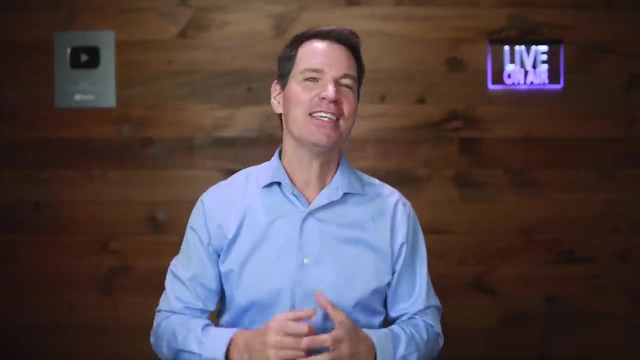 focus all your effort On your message and your audience. How can you best help your listeners? Focus on how to sharpen your message, the examples, the stories. so the message is the best it can be, And this is what great coaches and teachers do. If they share an example that doesn't go that well, they don't. 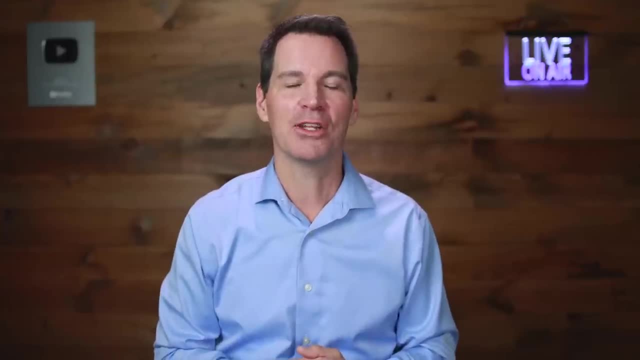 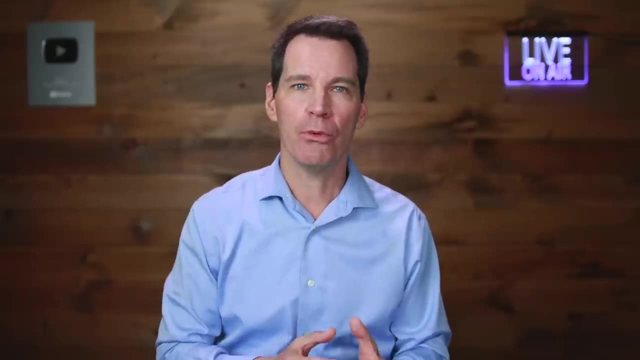 take it personally. They don't focus on them. They just move on and look for another example that will resonate with listeners. So focus on your message and helping your listeners to learn what they want and if that doesn't work, focus on that courage. 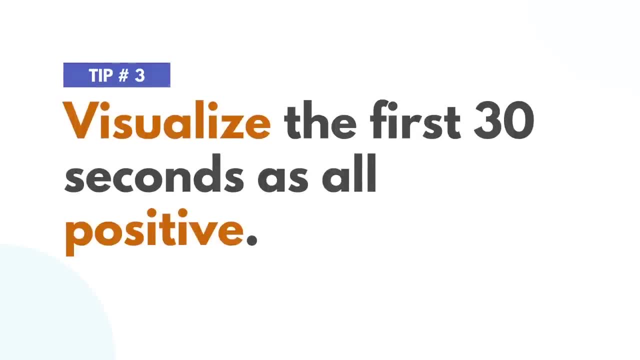 If you're a coach, you're not a student. You're not going to have the courage to start speaking out in front of them and really get their attention and attention. Think about that as something that will resonate with your audience and be there for them. 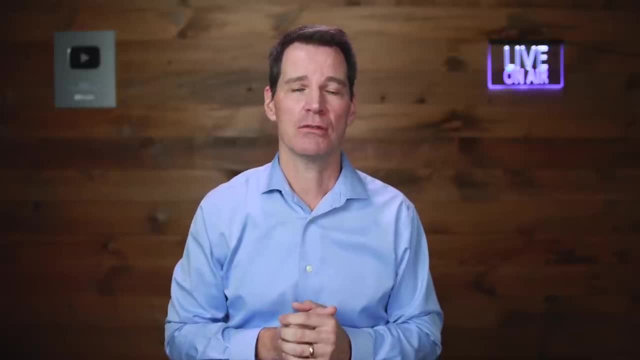 And see what LEADER has to say. You want to be there as a leader of the community and for your audience. You want to be a leader of the community and help your audience to understand this. You want to make the audience feel that you care about them. 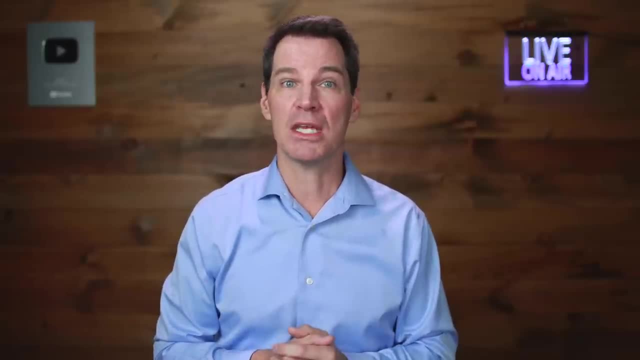 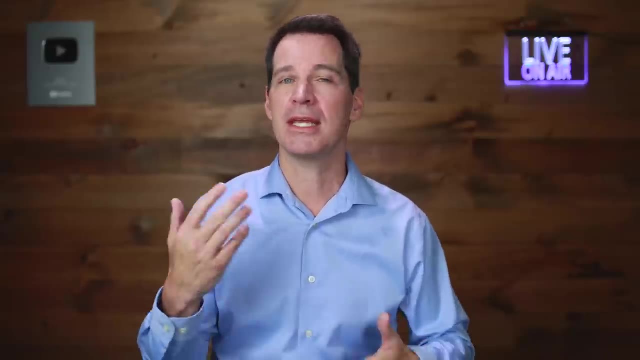 You want to say, the first thing you have to do is love them. That will make them feel comfortable. That will make your audience feel like they're in this group. You want to make your audience feel like they're in this group. That will make them feel like they're your friends. 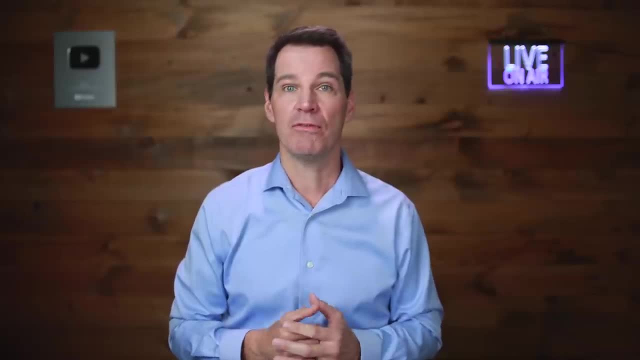 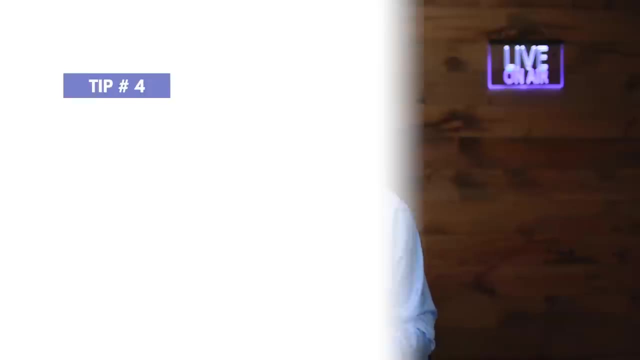 a positive way over and over again. This helps me feel good about the beginning, but it also helps me start on the right foot, because visualizing is another way to rehearse Number four- and I love this one- get there early and walk the room. 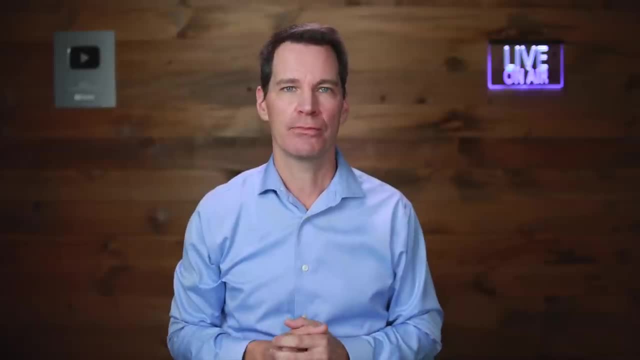 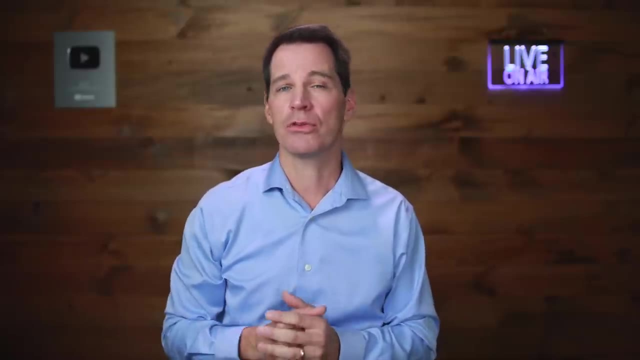 I always arrive early and walk around the room before it's full. I walk up and down every aisle. I look at the stage or the podium from the empty seats, then I stand in the front of the room or at the podium and I size up the room. 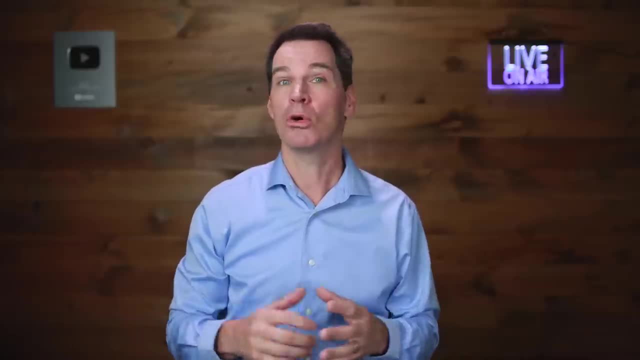 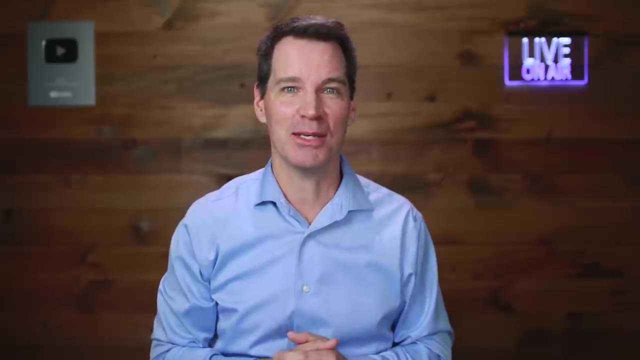 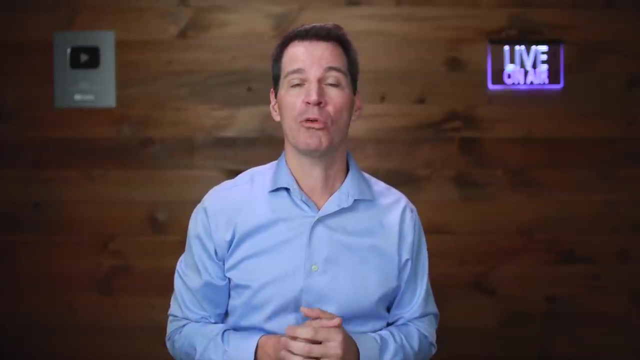 This makes the whole event seem smaller, somehow, and more manageable. I've heard that many professional athletes walk through the seats in the stadium when it's still empty before a big game. This will make the space feel like familiar territory. I spend a few moments at the podium or on the stage. 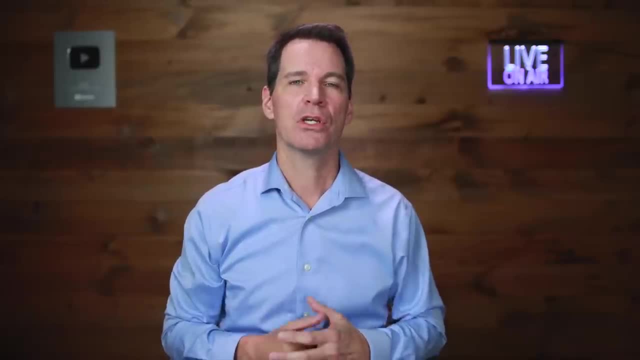 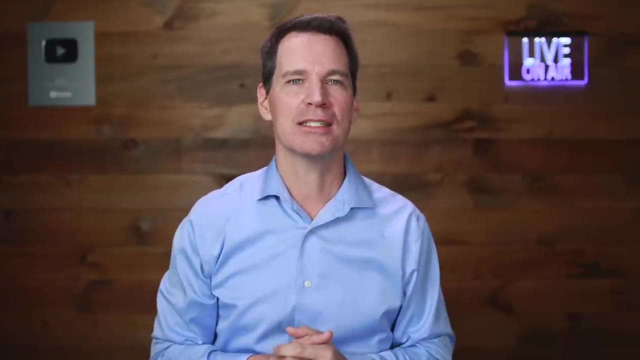 and again I imagine or quietly rehearse how the first few sentences will come out of my mouth and where I'll stand. This one tip: walking the room like this takes only about two minutes and always calms my nerves by at least 50%. 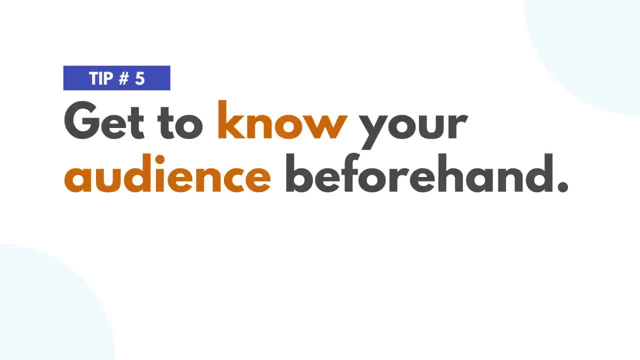 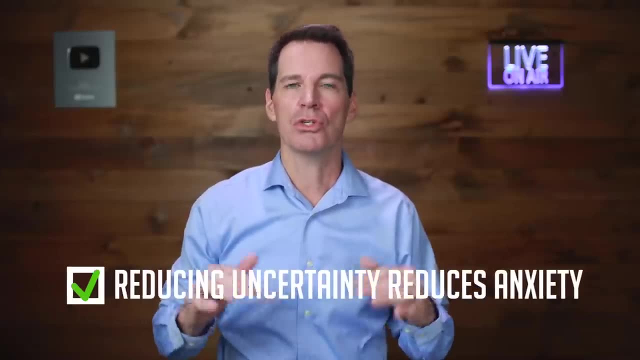 Number five: get to know your audience beforehand. Learn everything you can about your actual audience, the real people who are gonna be there. Reducing our uncertainty reduces our anxiety, And if I have a list of attendees ahead of time, I learn as many names as I can. 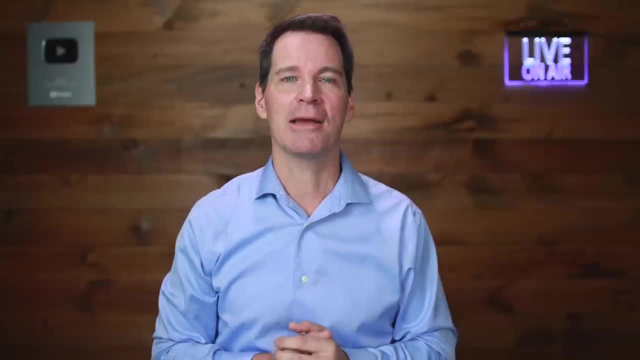 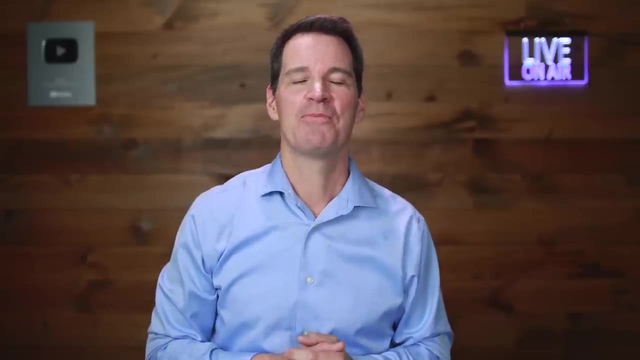 I also mingle. before any presentation. I shake some hands, I break the ice and make small talk about their backgrounds. I take a genuine interest in the people. This helps me feel like I already have some people I know and who are on my side.